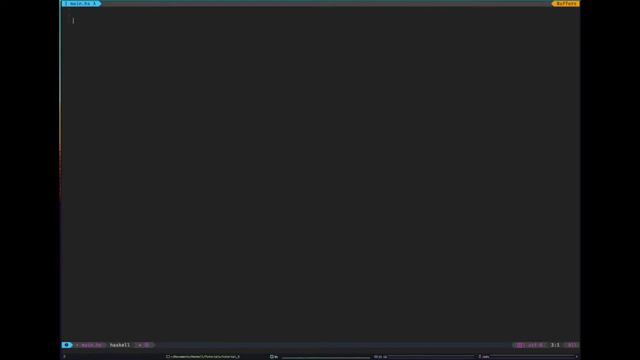 I think I will actually go into the file for this. So there's three ways to define types in Haskell. We're going to cover two of them in this tutorial. The first is the simplest: Type Type just makes type aliases. So I could say type id equals int And that's going to mean that 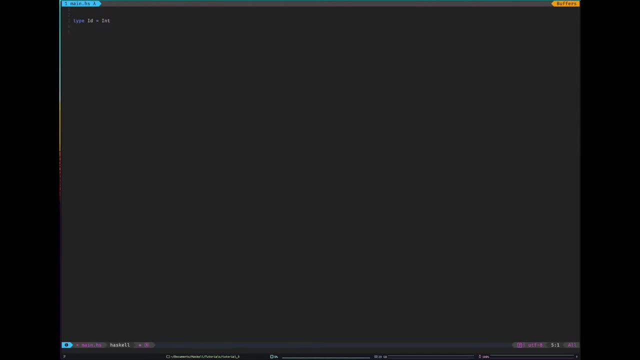 I could define a function that is int id to id. I don't know what it is, I don't know Map IDs, And it is a lot easier to sort of understand what that function does because I have given it id in its type name. So an example would be: 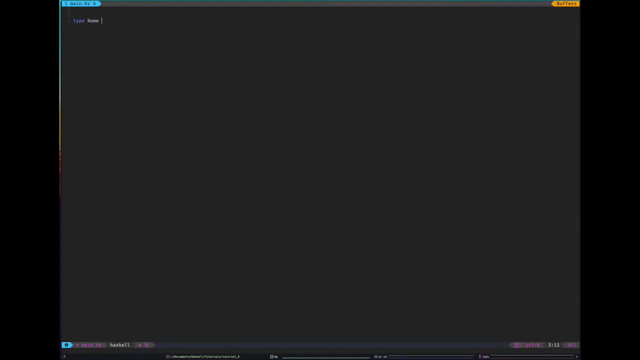 maybe another example might be: I could call it a name And that could equal string, And then type date of birth equals, and then a tuple, int, int, int, and then I can maybe write type, find, date of birth, and that would be of type name to date of birth. 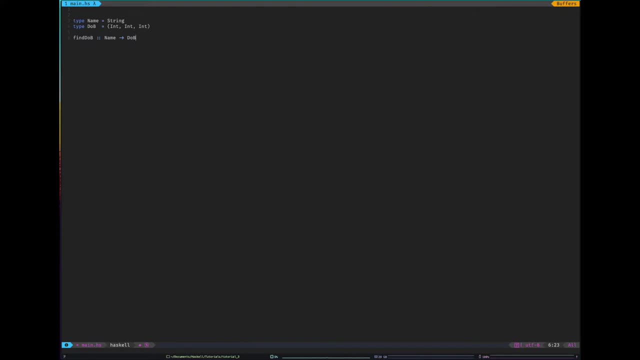 So you can see quite clearly there exactly what that function will do from the types. That's their first way of defining types. The next way, the more interesting way, is sort of building types from scratch, And to do that we use the data keyword in Haskell. 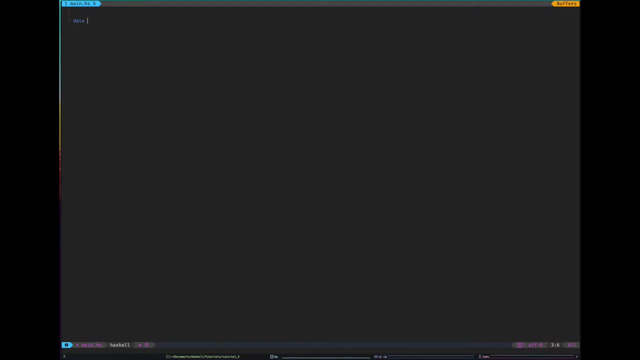 Now you know what is a type in Haskell? Well, Haskell has both product types and co-product types, or some types as they're sometimes called. So it's almost like type logic, if you like. co-product types. 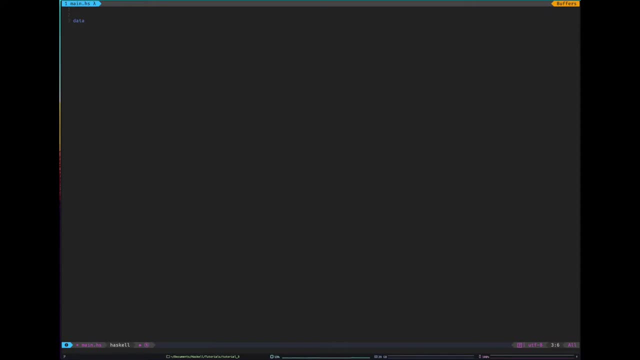 And you use this to describe what something is. That's how you think about types: What is something? So, for example, a list, say I wanted to redefine list in Haskell, I'd say: data list equals say it's just a list of integers for now. 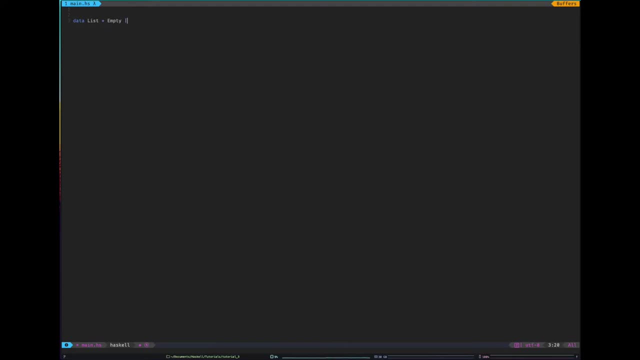 It's either empty or it's cons, remember, and that's the join keyword: int to list, And that's perfectly fine. That is a perfectly fine Haskell data type there, So I could go. what is the type of empty? It's a list. 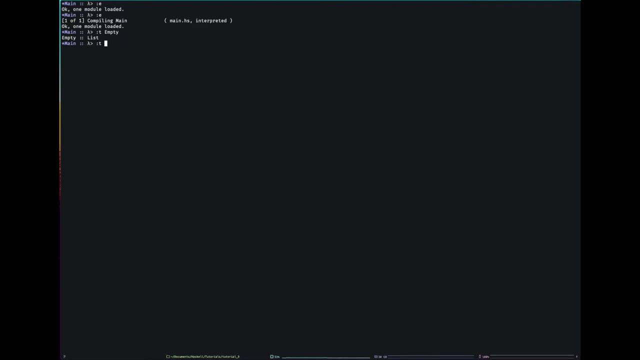 What is the type of cons? one cons, two cons, three cons, two empty. That's a list. That's the list. one, two, a linked list. So you really think about what things are when you're defining types in Haskell. 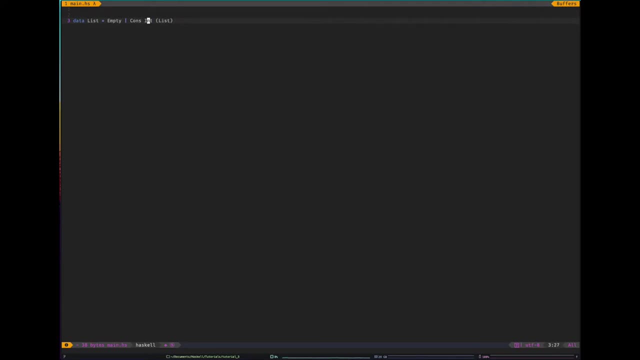 Now that's not a very good list. It only deals with integers. So in Haskell we can add type parameters for Parametric Polymorphism. So if I say List A, lowercase a, that's scolded. that allows me to sort of parameterize my type. 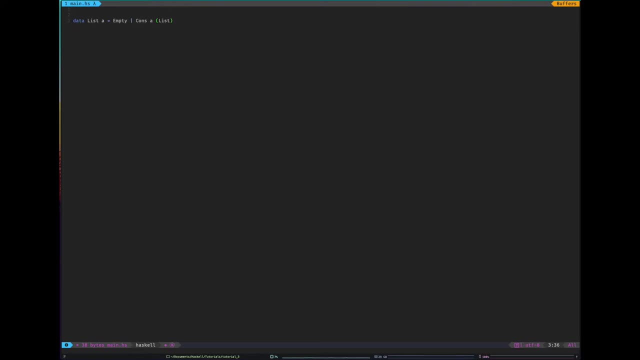 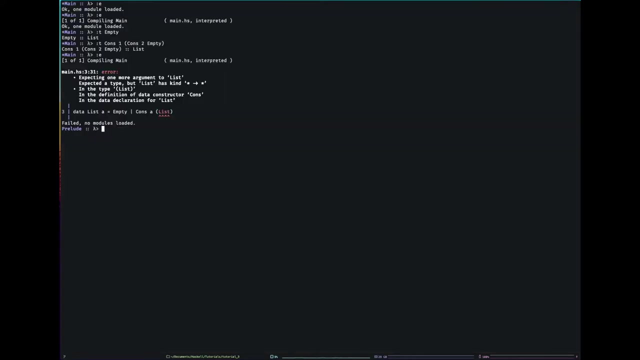 So I say it's not just a list of integers now, it's a list of type A, And you can see I adjusted the type definition accordingly. So now, oh, and of course I forgot to pass that back. list of type A. 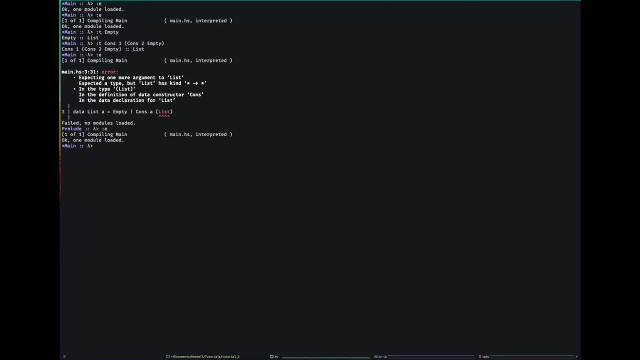 Perfect, So now I could go: okay, what is the type? of same one as before. So now it's a list of type A, where A is a number. We're gonna deal with this syntax later. Maybe a more sort of clear cut one would be. 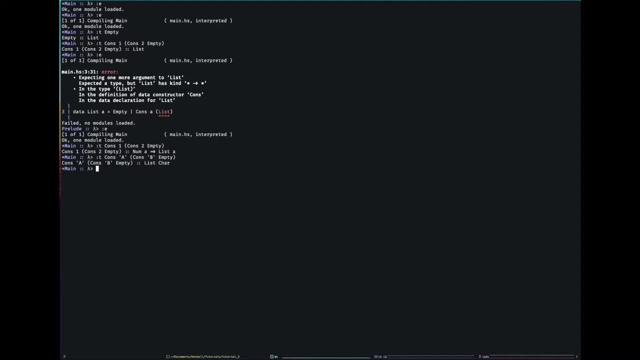 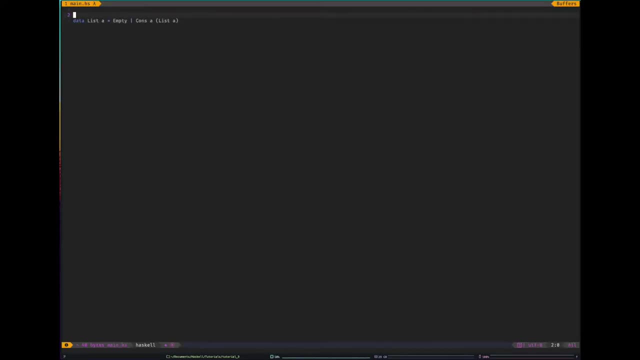 if I had A and B. Now it's a list of characters. Notice that that definition is recursive. I mentioned list A in the definition of list A. that's perfectly fine. in Haskell It's done very often when describing tree-like structures. 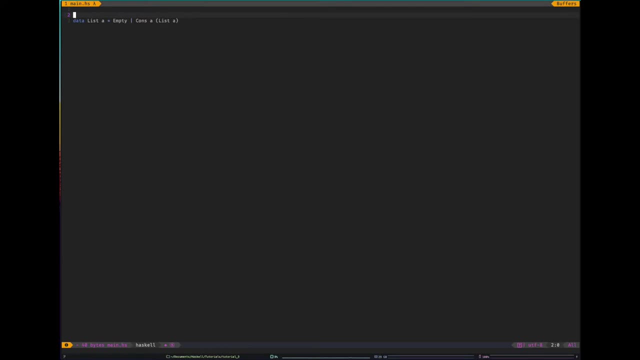 maybe or anything Cool. So the next thing is: how do we use these types? So let's make something that converts a list of the type we've made there to a normal Haskell list. So we'll say: to H list, Haskell list. 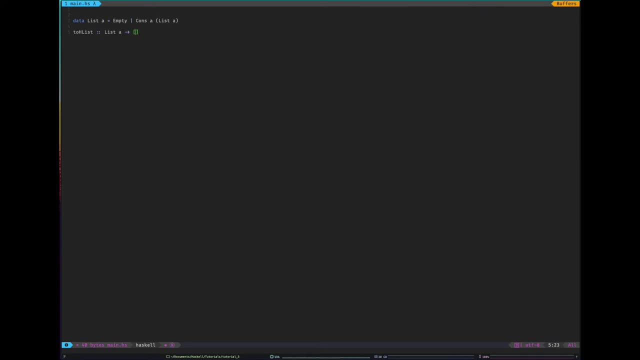 and it's gonna be a type list And it's gonna be of type list a, two, and then the haskell version of list two, h list, and now pattern matching these constructors- and they are constructors- um, we can kind of extract data from them when. 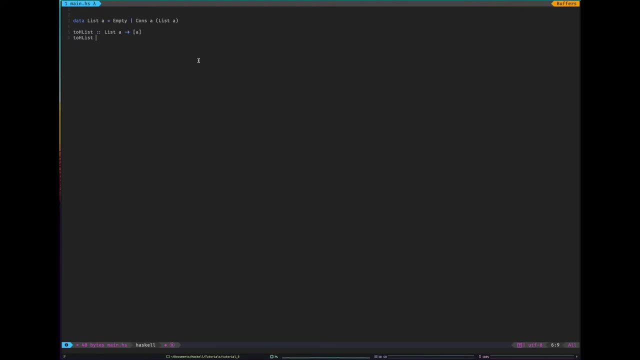 we define functions. so i'm going to say 2h list, empty, equals, and then the haskell empty list, 2h list, and then in brackets, cons x, x's equals. i need to align these things or else i suffer. is going to equal x cons x's in haskell format. now this is interesting that i've done. 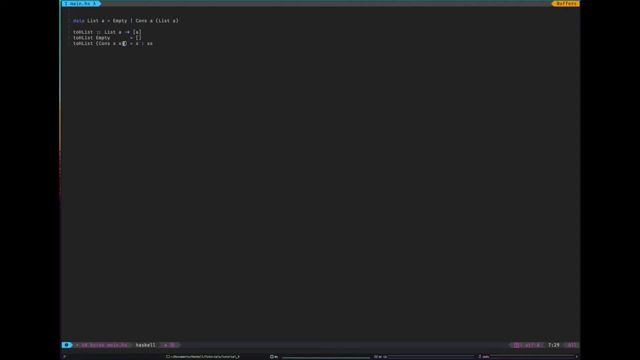 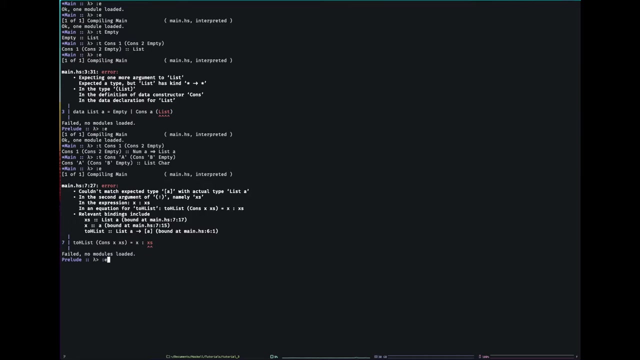 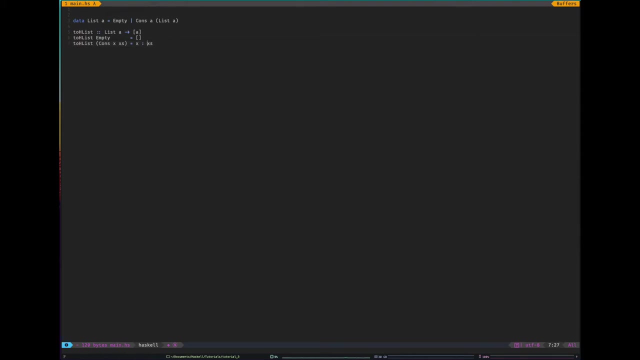 it like this: um, like this, sorry, this x's is matching this, oops, and that x is matching that in the type, and that's it. we, we kind of decompose types like that. um, oh, of course, so x's is not of the right type. i forgot, i need to recursively call. 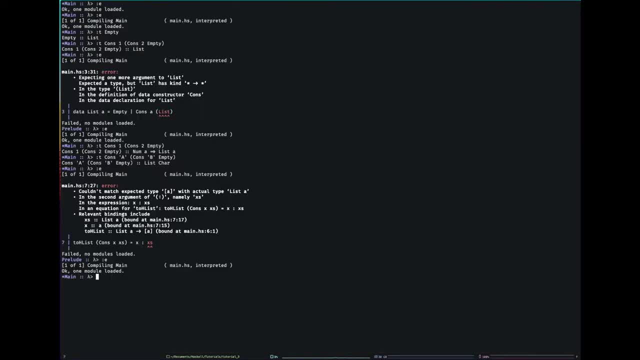 h list. there we go now it works. so i can go take that and i can say to h list and then, uh, dollar, and we have the haskell list equivalent. um, that dollar, by the way, is to avoid writing brackets. so if i took that dollar away, the way haskell would read this: 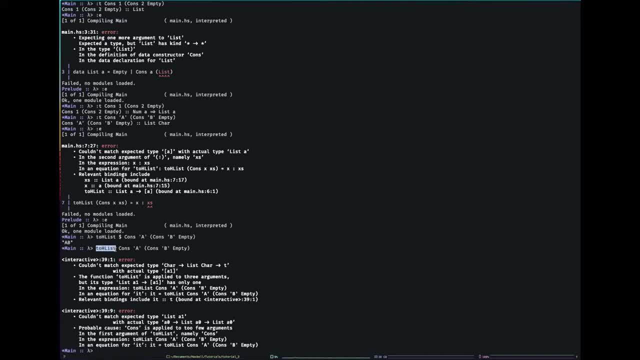 you'll see it's going to error. is it goes to list? okay, that takes in a list. next thing, cons. but that's not a list, that's a constructor, that's a function in haskell, so it errors. it was expecting a list, it got a function and it- um, it does say here somewhere: 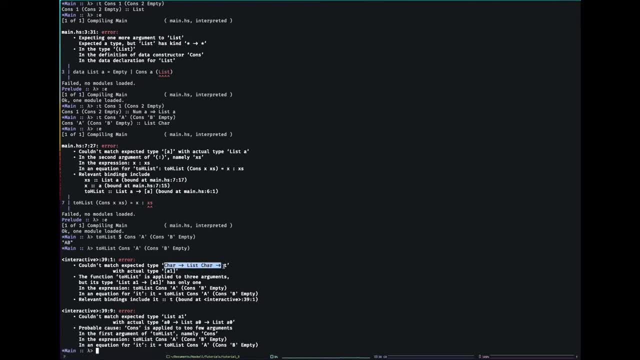 it couldn't match expected type charter list, charter t, which is the type of cons with. well, who knows, anyway it'll give me two errors. ah, that's better, couldn't it? that's what it expected: to get something of type list a1, but instead it got this. so 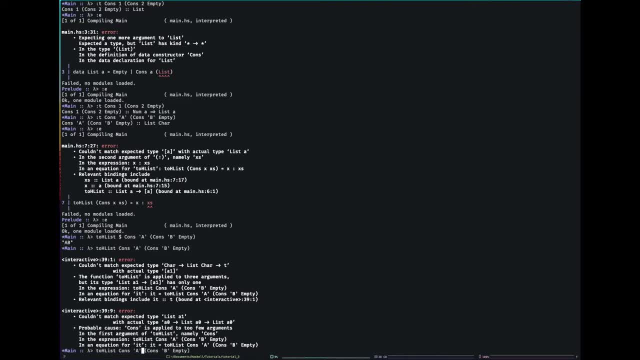 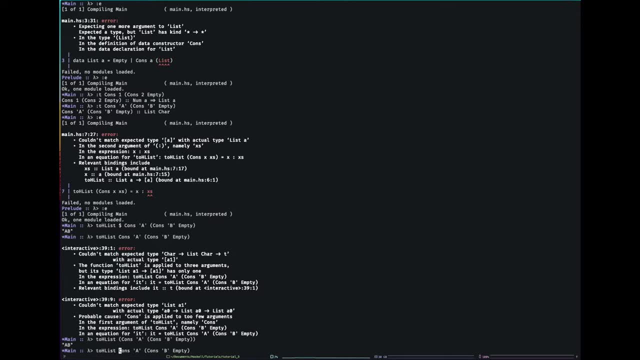 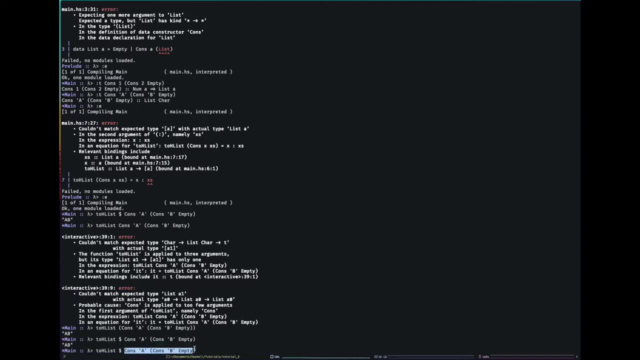 um, that dollar just allows, because i could fix that with brackets, but brackets are ugly, so, uh, sometimes it's better to just use the dollar, and what the dollar says is: calculate everything that comes after it first. okay, we're going to use that quite a bit. so, uh, good, and and now that you know about sort of parametric types or parameterized, 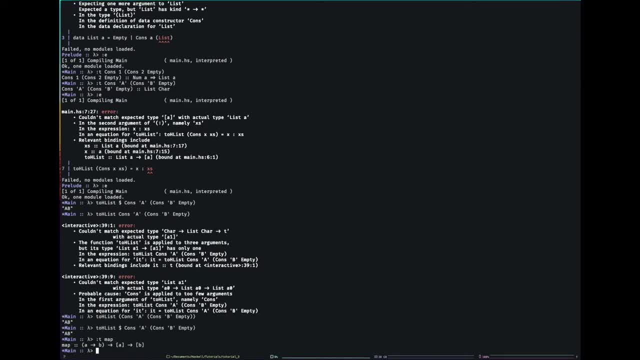 types. Types like map make more sense. You know, it takes a function of type A to B and maps that to a function- list A to list B- And that's quite cool. That's quite cool. So we've done pattern matching. Oh, so I should mention probably how to pattern match lists. 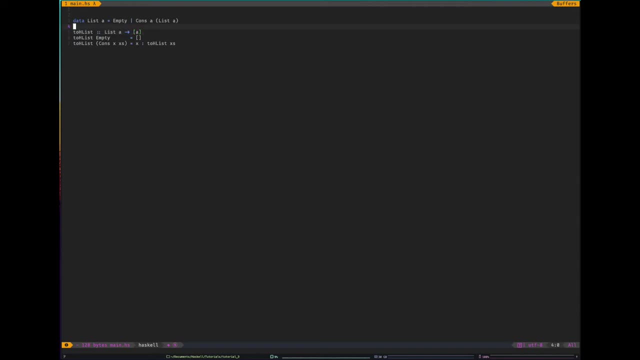 Um, it's kind of how you'd expect, So I could redefine map here, this time not using list comprehension, And I say: map of empty is empty. Map of x attached to x's equals. oh, I forgot. Map takes in a function, fx joined to map fx's And um. 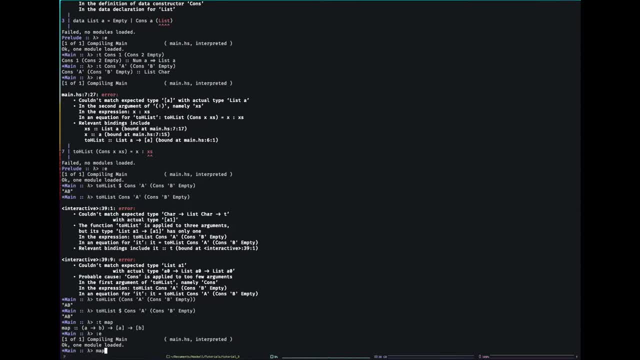 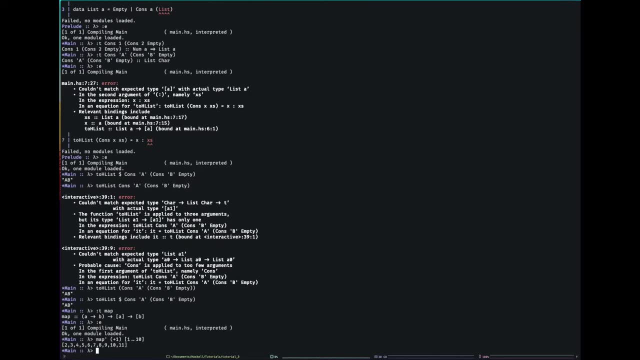 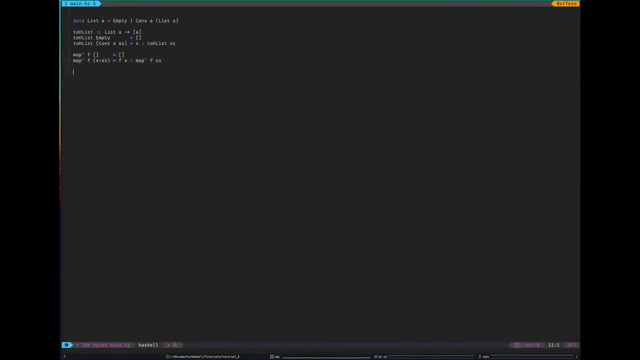 there we go. That's a perfectly good definition of map Um. same example as before, Perfect. So let's go back to type definitions. So I said you kind of think about what something is when you define the type. It's a bit like in um, it's a bit like when you're doing um. 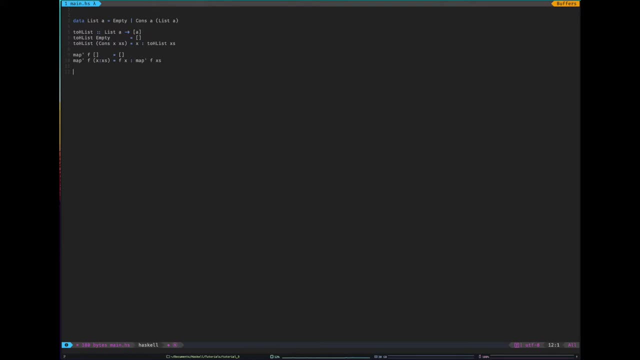 object-oriented programming, where you define types in terms of their functions. Um, you kind of call this in Haskell, adverb-oriented programming. Anyway, it doesn't matter, Doesn't matter? Um, let's think of a good example. So let's encapsulate error handling. 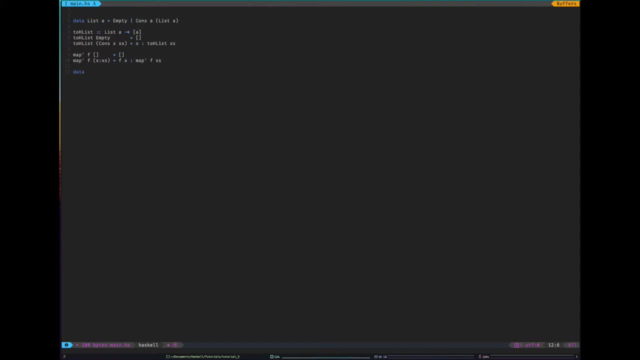 So we're going to make a type called um error and it'll be a type A And it equals: is error a good name? Because it's kind of, it doesn't matter, And it's either going to error. 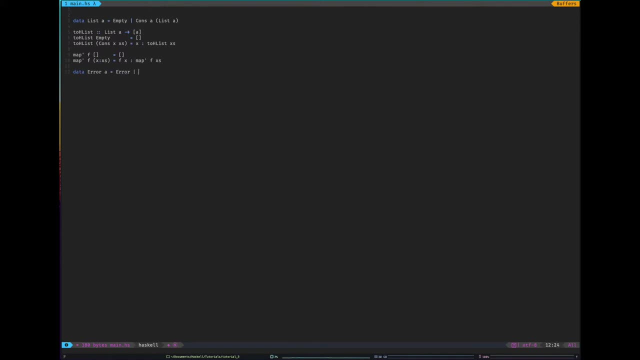 or it was okay and we passed the A, So this is, this is interesting. Um, what can we do with this type? So let's make a safe divide function. Safe divide function. So what this is going to take in is this is going to map error. 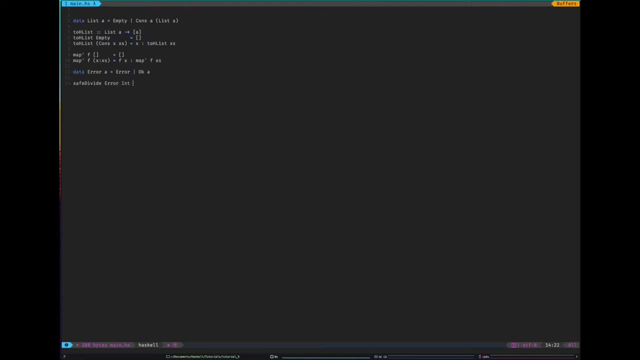 Int to error, int to error int. And essentially, if we divide by zero at any point, we will error And if we don't divide by zero at any point, it'll be okay. of the answer, So safe divide. First of all we need to check, and this is going to be quite clumsy, but I'm 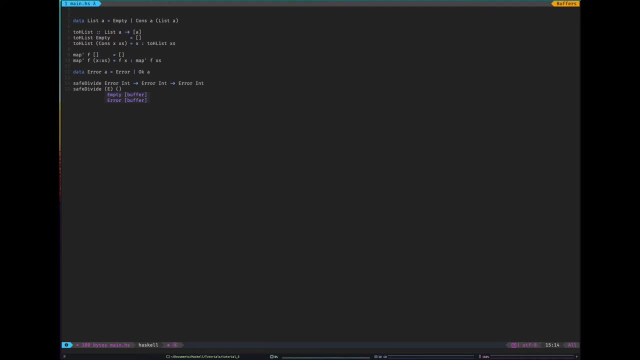 going to show you different constructs later on. So we're going to check, and this is going to be quite clumsy, but I'm going to show you different constructs later on That'll allow you to really simplify this. So an error x? um, no, no, sorry, sorry, sorry, sorry. 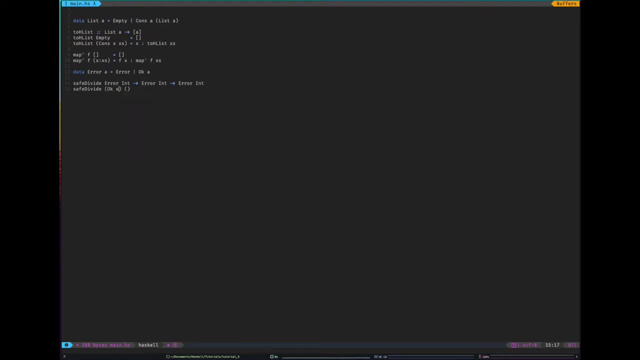 pattern matching. So okay, x, Um, no, actually I will go back to how I did it, So we'll start off with the error terms. So error. if the first thing is errored, we want to return error. 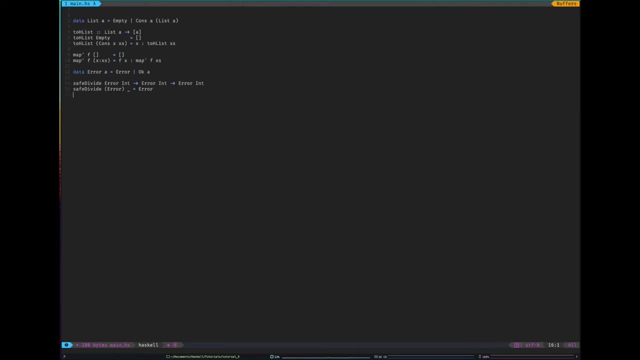 So what this underlist score does is it means we're just going to completely ignore whatever's there. Um, we're then going to do exactly the same if the second thing has errored instead, Um, cool. But then if neither has errored- okay a, okay b, then we can do: um, okay. 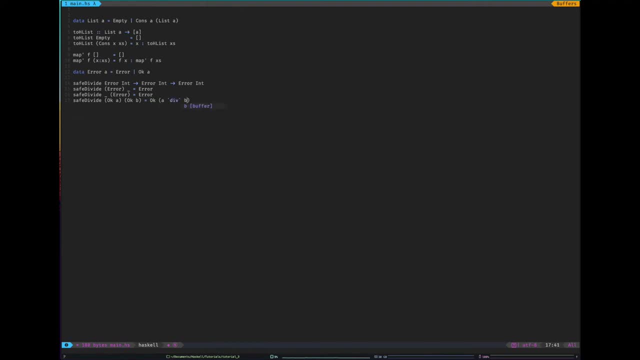 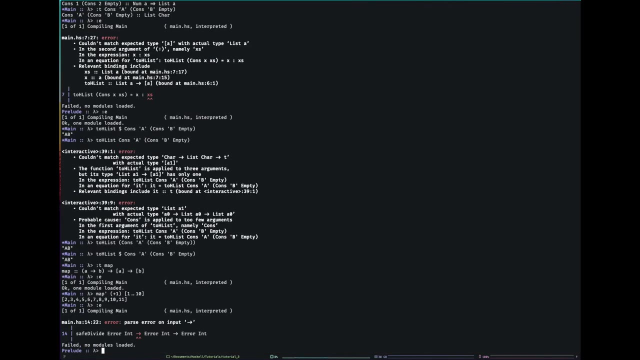 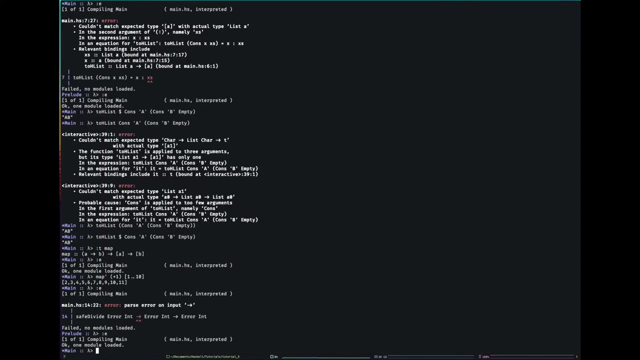 a div b And you see we're kind of extracting the value of a from there and b from there. So oh, I forgot a bit of syntax there. Perfect, So we can try and test this out. But first of all, 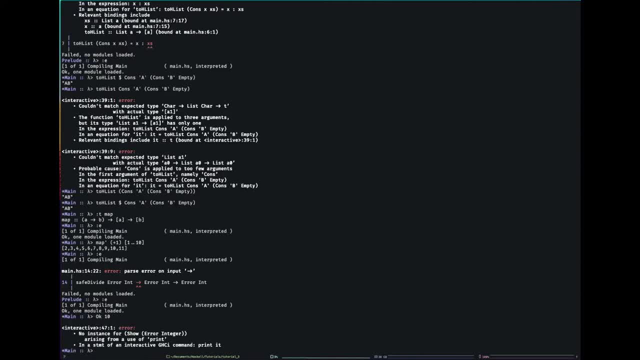 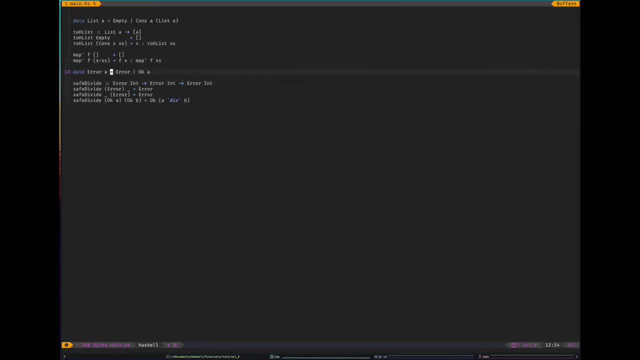 if I just say okay, 10, it's going to error. It says no instance for show. Basically, Haskell doesn't actually know how to print. I'll type out on the screen, but we can fix that. And next tutorial I'm going to go into. 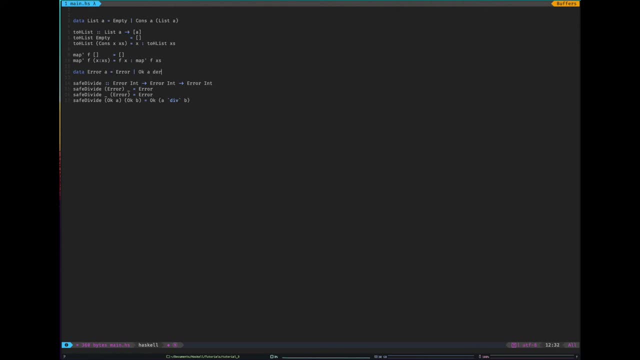 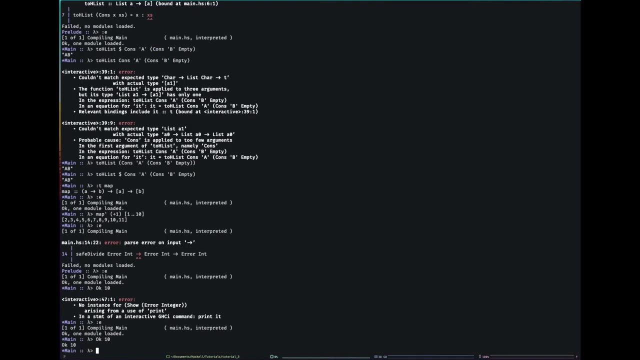 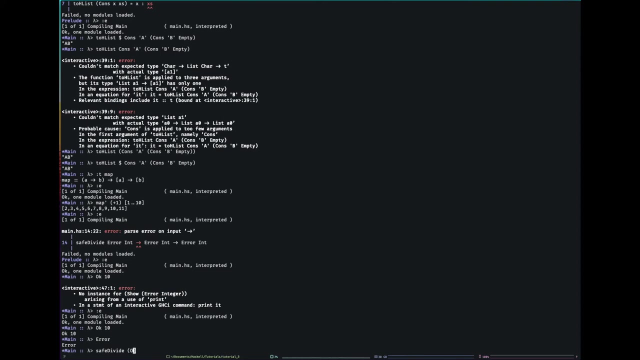 what we're doing here. but I can say deriving, and then show. Now it knows how to print out our types. So there we go. Okay, 10 or error, And then we can do safe divide. Okay Five, Okay Two. 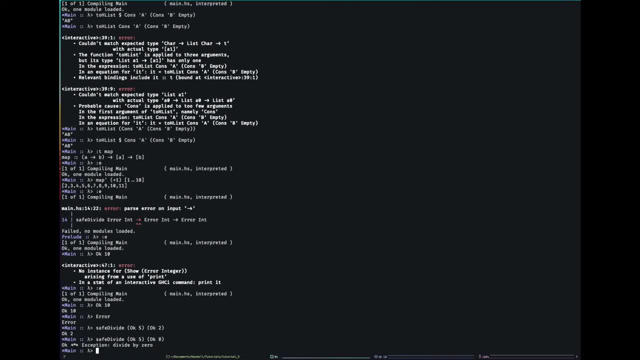 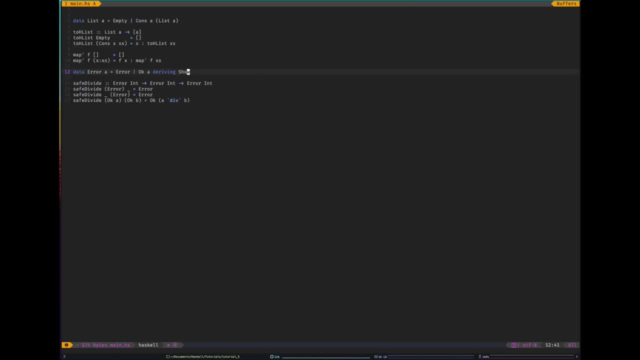 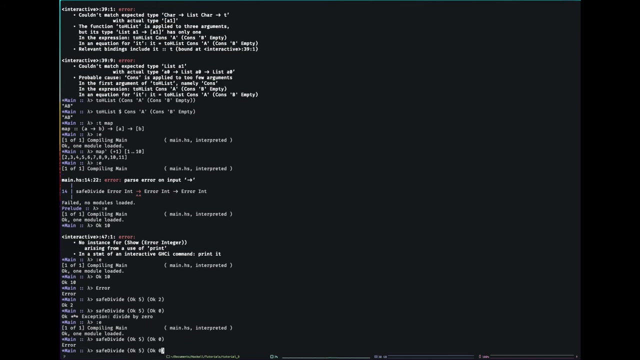 Okay, But if I do zero, Oh, I can't do okay, Zero. Um, let me say what I'll do is I will go like this: Um, my apologies, I forgot the actual safe bits. There we go, I'll try that again. Error, And if I try and safe, divide that by something normal. 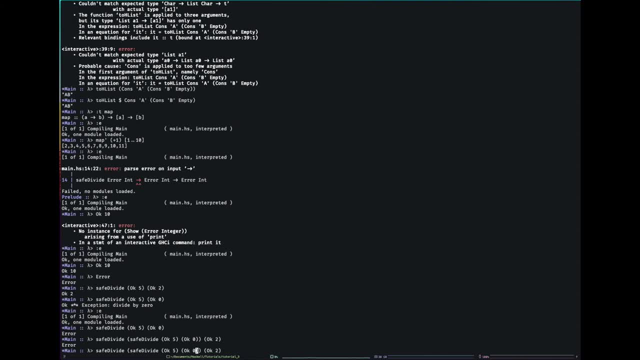 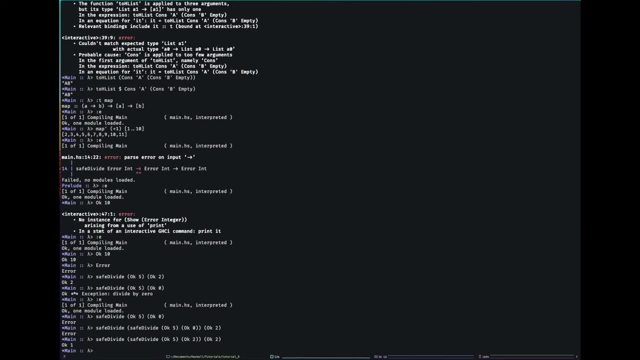 it's still going to error. I have to make that not error first. So this is kind of a way of doing error handling safely in Haskell instead of getting a horrible exception like the one we got: exception divide by zero. So I'm going to do safe divide And if I do zero I'm going to say 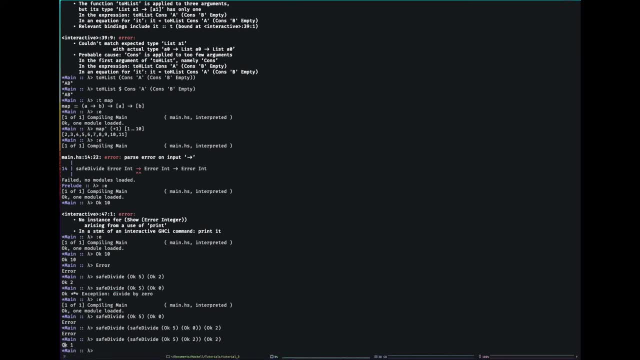 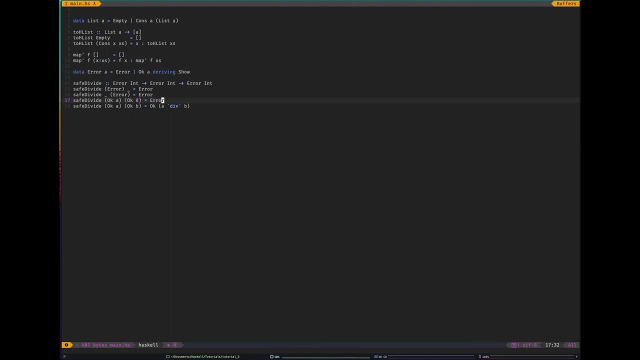 zero Um, we get a Haskell type back that we can reason about and we can do error handling in the code itself. So I think it's quite an elegant way to deal with um error handling. So we've done pattern matching, We've done sort of thinking about building types. Let's go for there's. 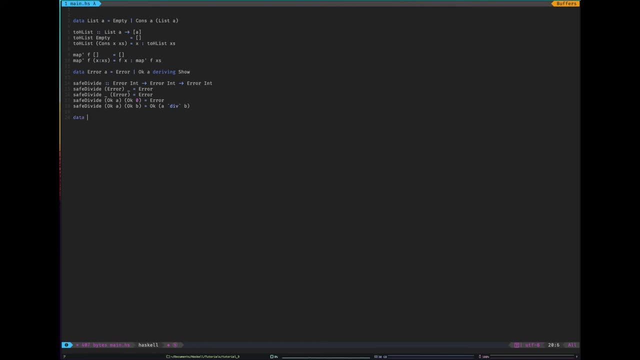 so there's another type of syntax. Um, so it's quite a clumsy way of making something. it's not a good way, so far, of making something like a struct in haskell, because i could say, okay, date a person, and then a person has a name, an id, a date of birth.